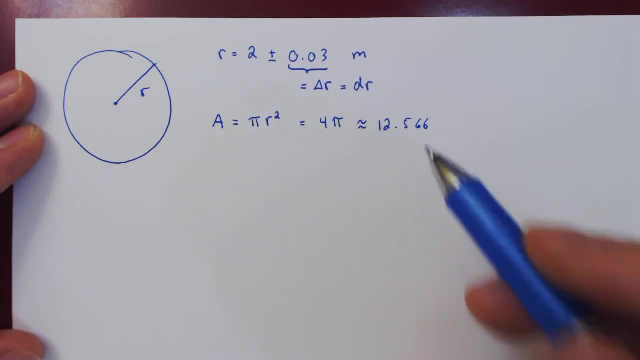 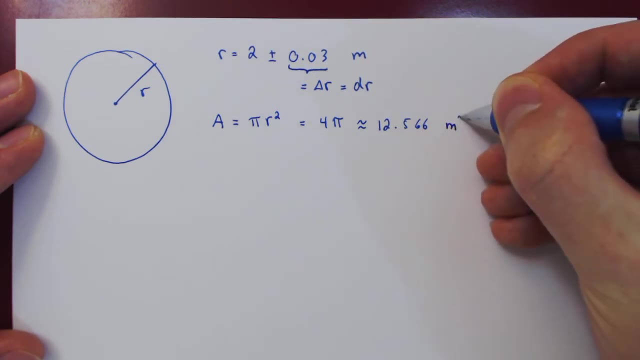 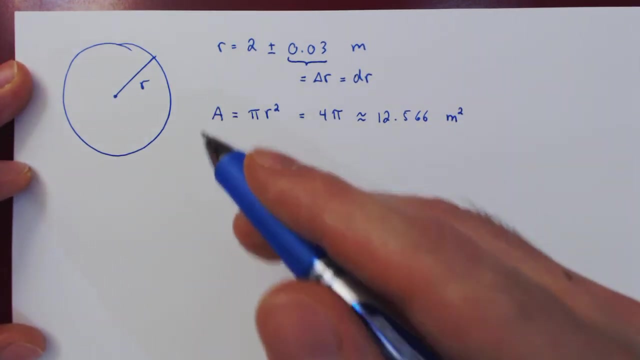 So that was the easy part, right. We now have the area of the circle to be approximately 12.566 meters squared. And how do we now find the uncertainty of the area? Well, the uncertainty in the area will be a small change in the area, namely delta a. 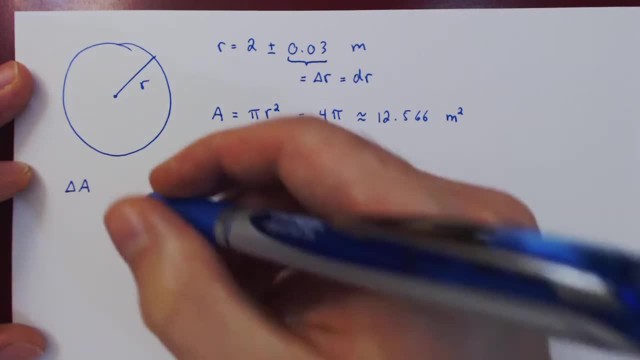 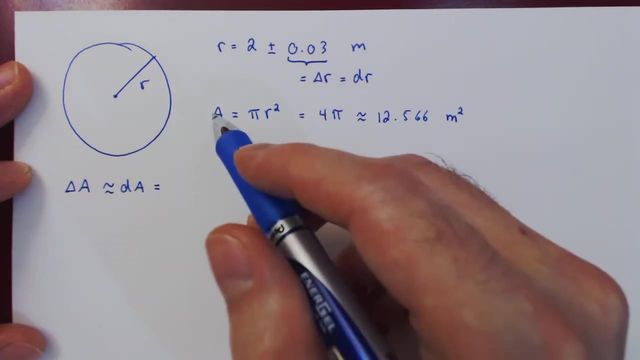 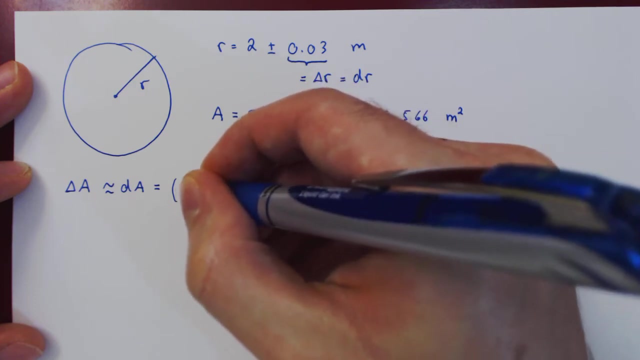 And now, of course, we can approximate the change in the area by the differential in the area dA. And of course, the differential of a function, where now here a is a function of r, is given by the slope of the function with respect to its independent variable. 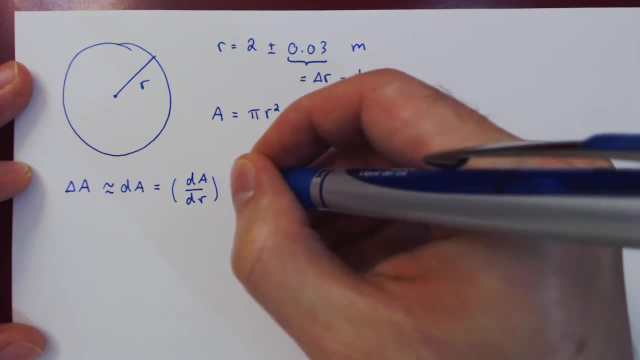 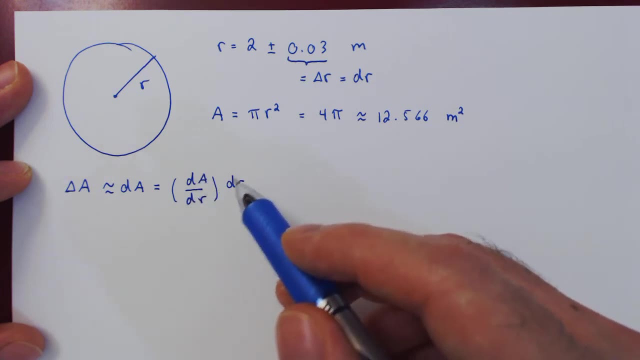 so the derivative of a And the derivative of a is a function of r, which is the value of a with respect to r, of course, times the change in the independent variable, the change in r, And it's clear that dR and dR cancel and we get, of course, dA. 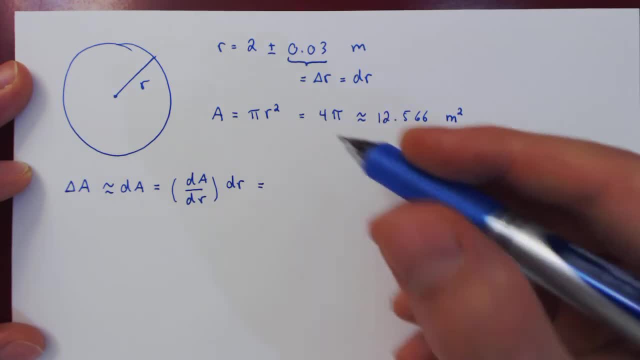 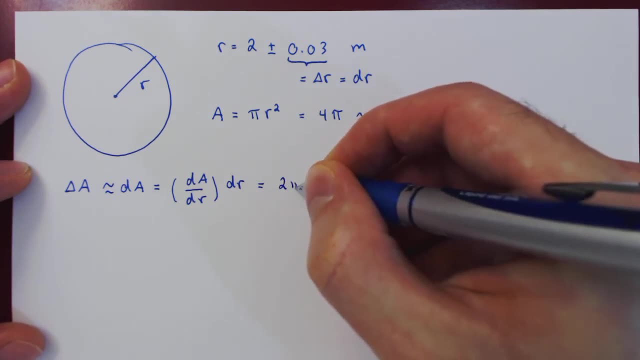 So now let's differentiate a with respect to r. So pi is a constant multiple. This will give us, by the power rule, 2 pi r times dR. And now we have a constant multiple and we can calculate it by the power rule 2 pi r times dR. 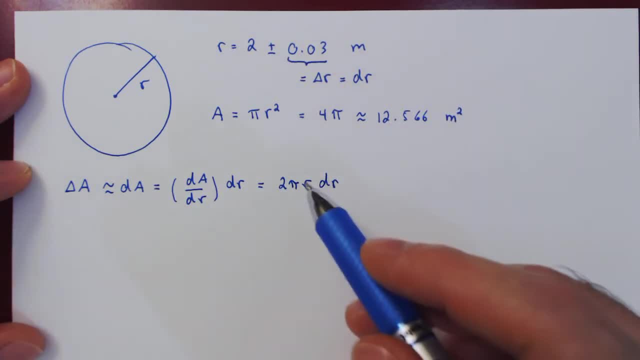 And now we have the differential of the area for any value of r and any change in r. So we can now evaluate: The value of r is 2, so we have 2 times 2,, 4 times pi, so 4 pi. 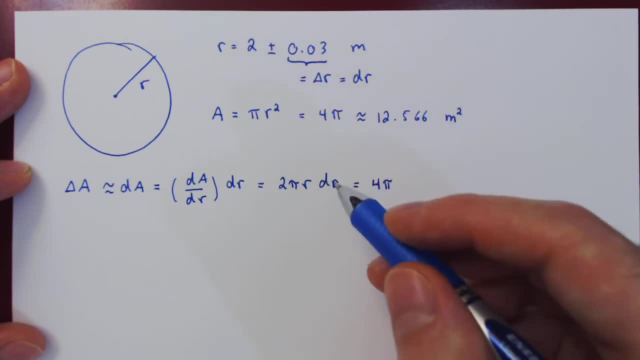 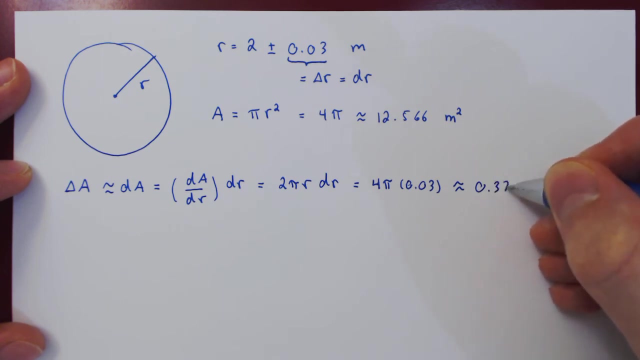 times the differential in r, the change in r. that is of course the uncertainty 0.03.. And if you multiply this out, you will obtain approximately 0.377 meters squared. And now we can write down our conclusion. 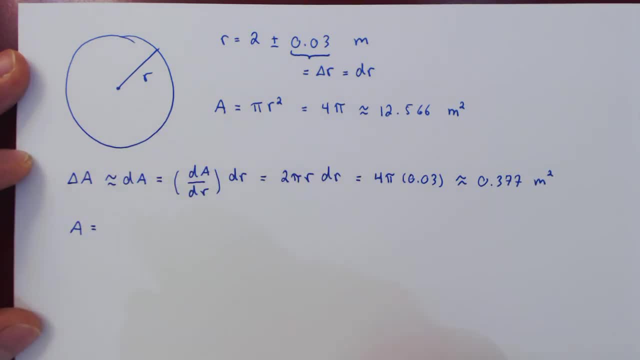 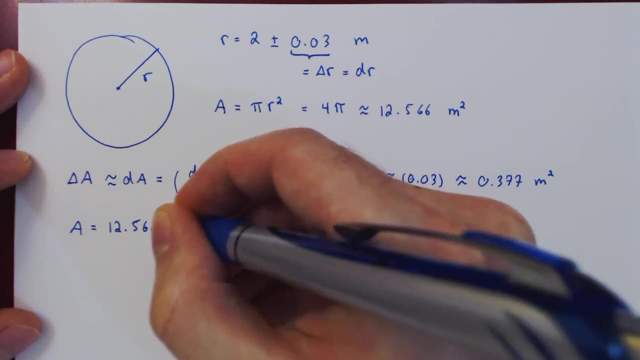 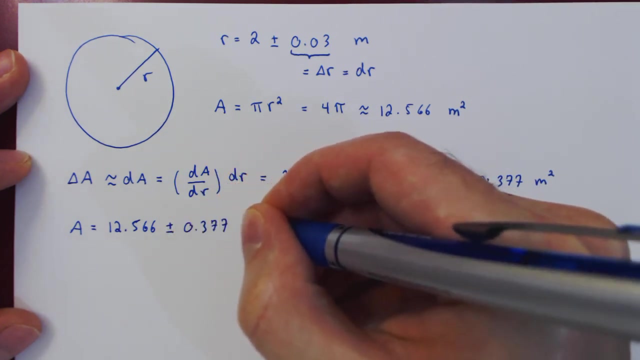